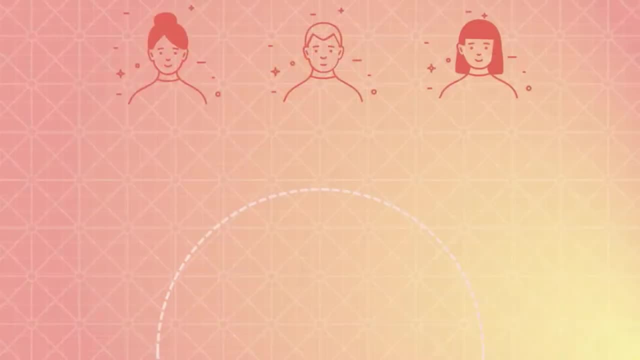 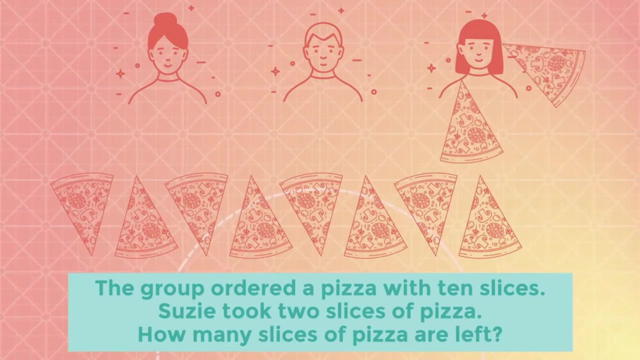 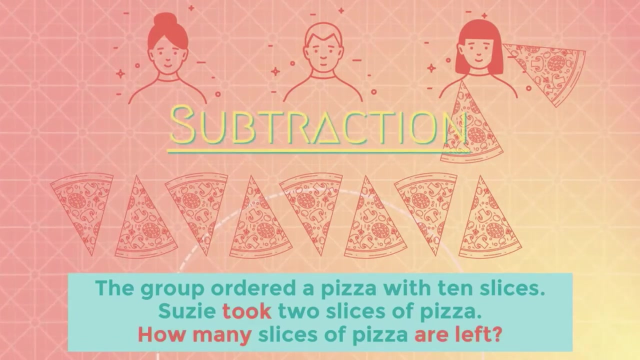 are used often for certain types of operations. Let's look at an example. The group ordered pizza with ten slices. Susie took two slices of pizza. How many slices of pizza are left? Which words or phrases are clues Took and how many are left? These words imply subtraction And because we started with ten and took two. 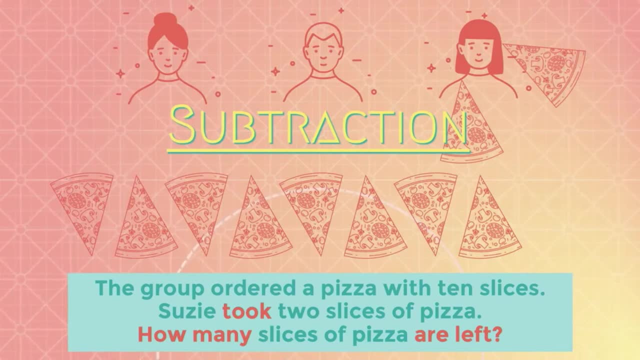 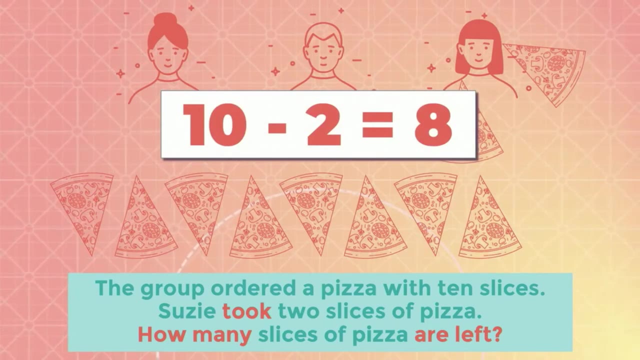 away. we can guess our answer is going to be smaller, which confirms we should use subtraction. In this case we'll subtract Susie's two from the whole ten for a difference of eight. Let's look at another situation. Professor Salmon needed to order two notebooks for each. 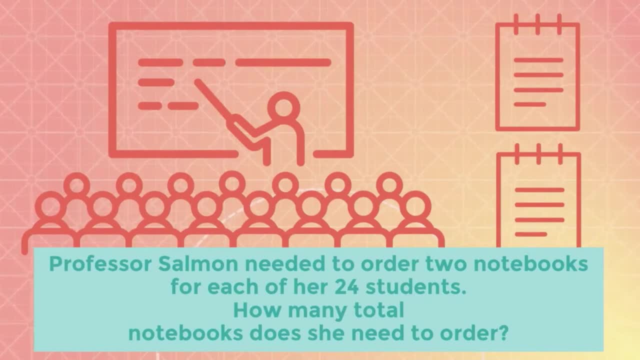 of her twenty-four students. How many total notebooks does she need to order? Can you find the clue words here? How about for each and how many total? These words imply that our answer is going to be larger than the parts of the equation, Because we know we. 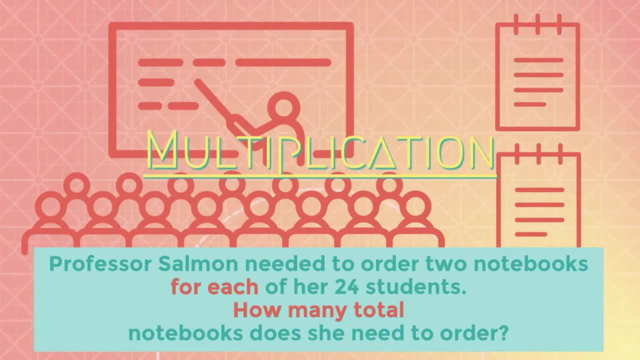 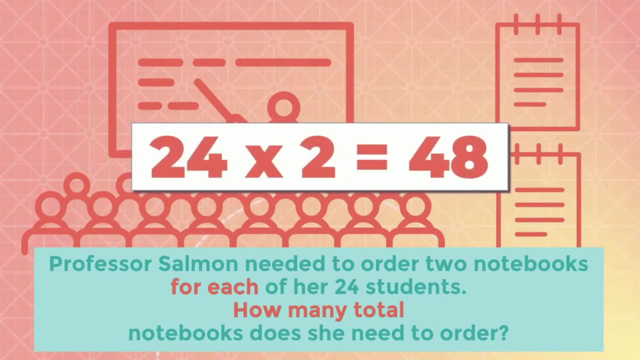 need two of something twenty-four times. we can determine the best operation is multiplication. Twenty-four times two is forty-eight. Professor Salmon needs to order forty-eight notebooks. Let's look at some other signal words that might help you determine the operation needed. 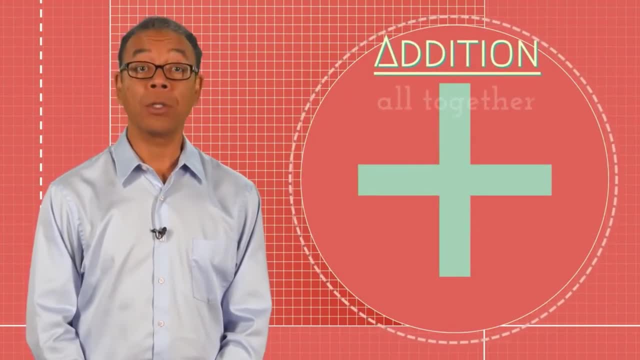 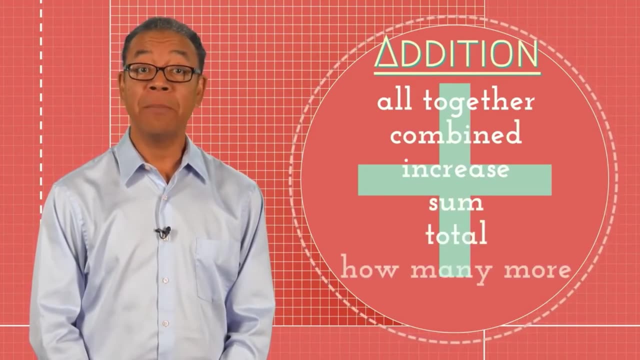 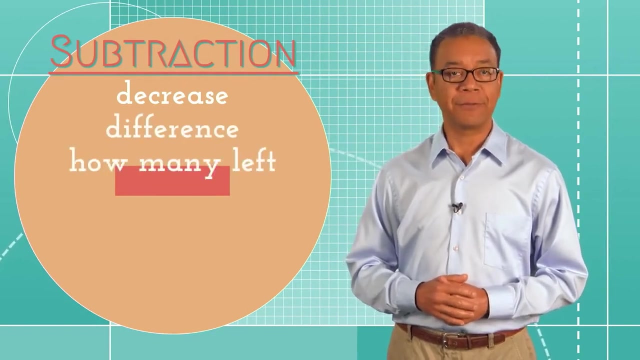 When you need to use addition, you'll likely see words such as all together combined, increase, sum, total and how many more. For subtraction, look for words like decrease, difference, how many left remain, take away and how many. 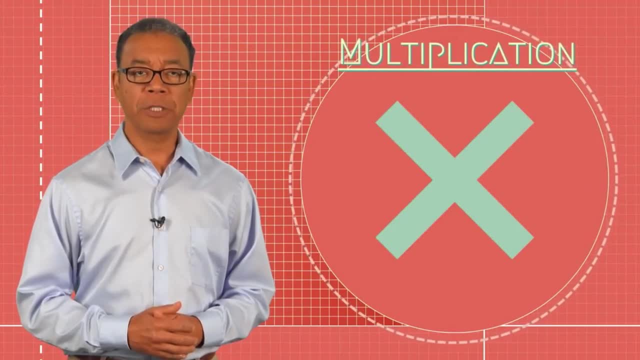 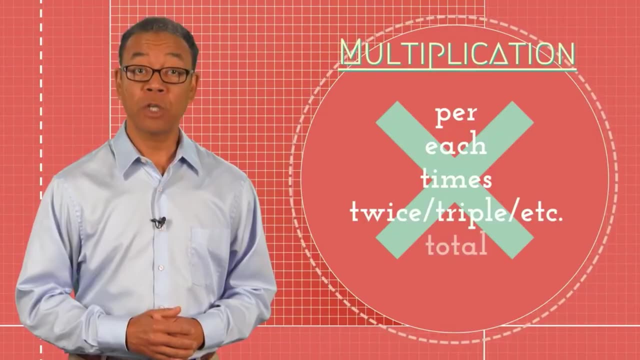 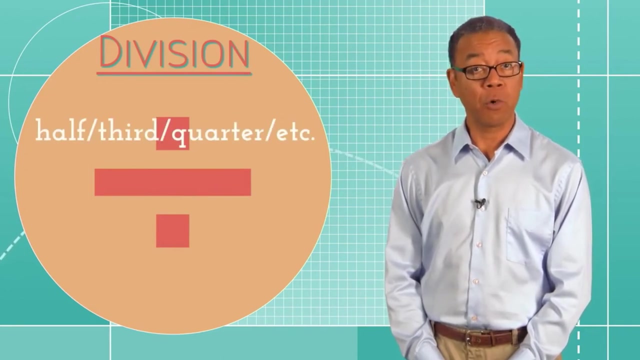 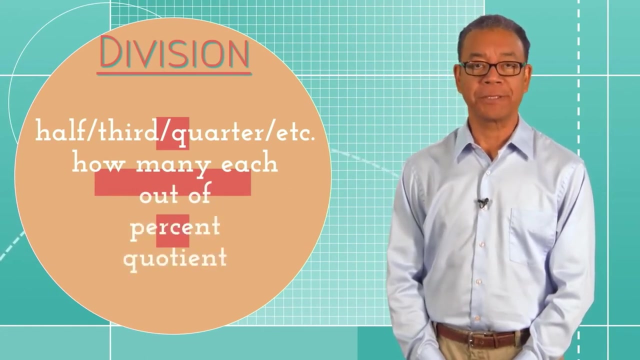 many more than For multiplication, you'll find words like per, each times twice, triple, etc. and total. And lastly, for division, you'll want to keep an eye out for these words: half, third, quarter, etc. How many each out of percent and quotient Knowing. 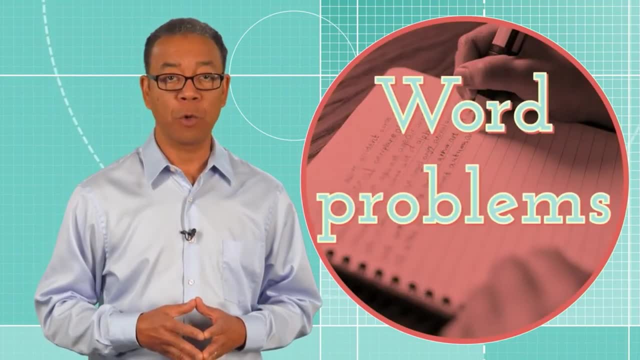 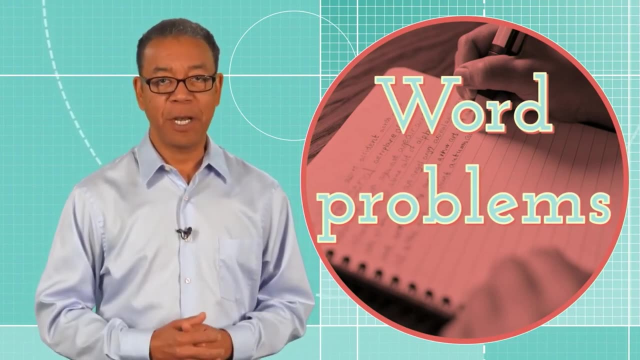 how to choose the right operation is a key part of solving word problems and dealing with math in practical, real-life situations. Knowing these signal words and strategies will help you successfully choose the right operation to solve any word problem that comes your way. 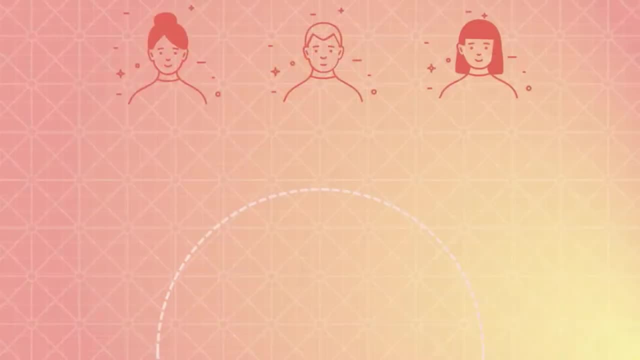 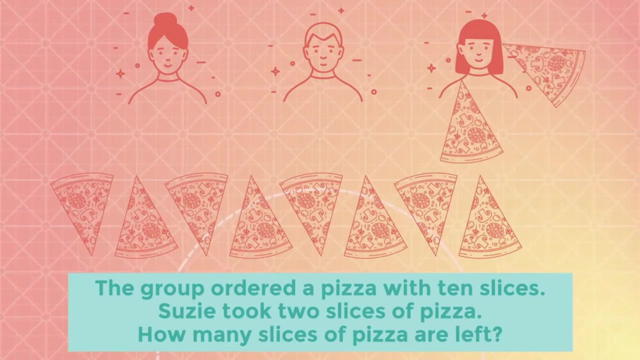 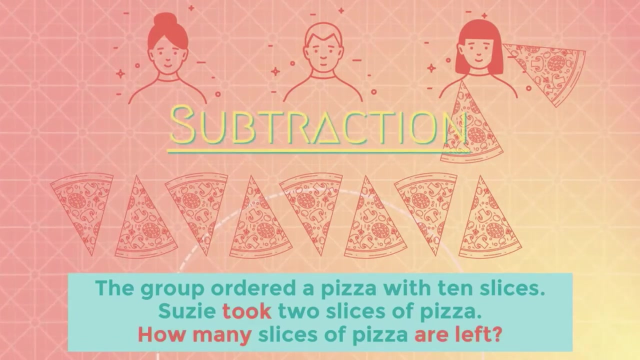 are used often for certain types of operations. Let's look at an example. The group ordered pizza with ten slices. Susie took two slices of pizza. How many slices of pizza are left? Which words or phrases are clues Took and how many are left? These words imply subtraction And because we started with ten and took two. 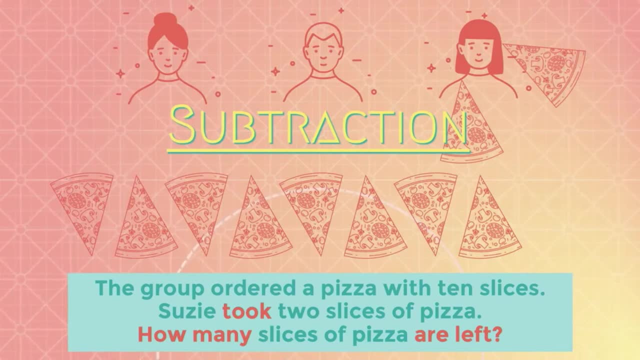 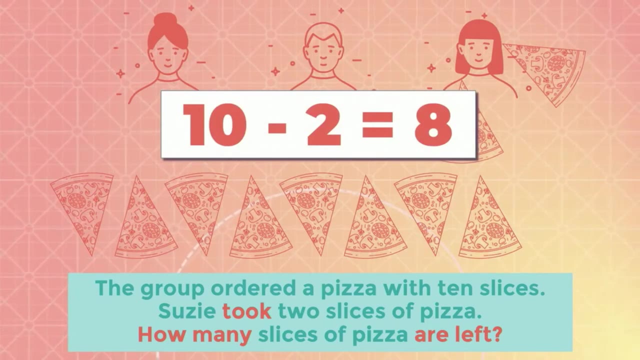 away. we can guess our answer is going to be smaller, which confirms we should use subtraction. In this case we'll subtract Susie's two from the whole ten for a difference of eight. Let's look at another situation. Professor Salmon needed to order two notebooks for each. 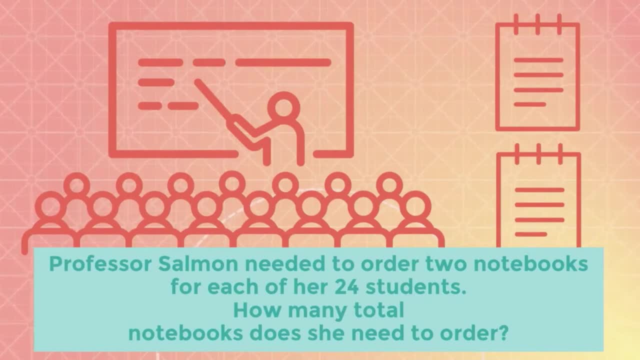 of her twenty-four students. How many total notebooks does she need to order? Can you find the clue words here? How about for each and how many total? These words imply that our answer is going to be larger than the parts of the equation, Because we know we. 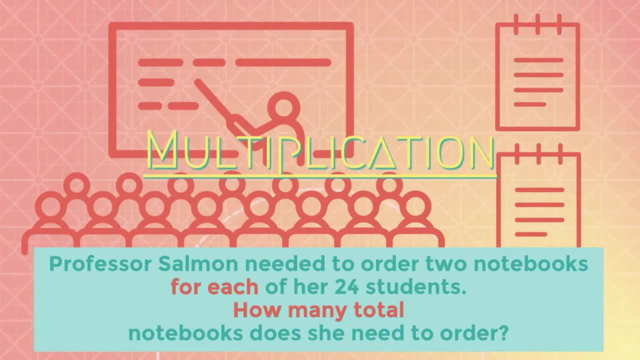 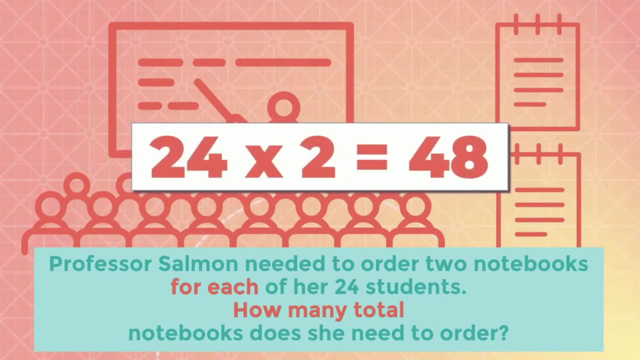 need two of something twenty-four times. we can determine the best operation is multiplication. Twenty-four times two is forty-eight. Professor Salmon needs to order forty-eight notebooks. Let's look at some other signal words that might help you determine the operation needed. 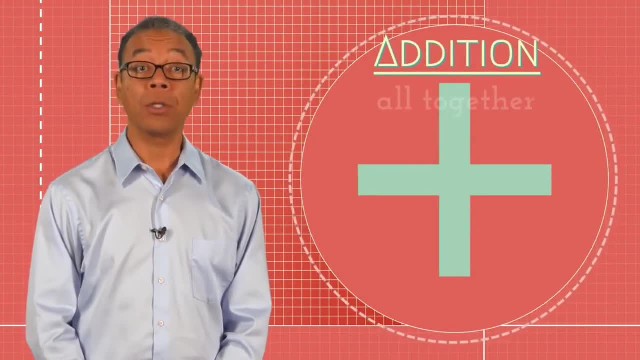 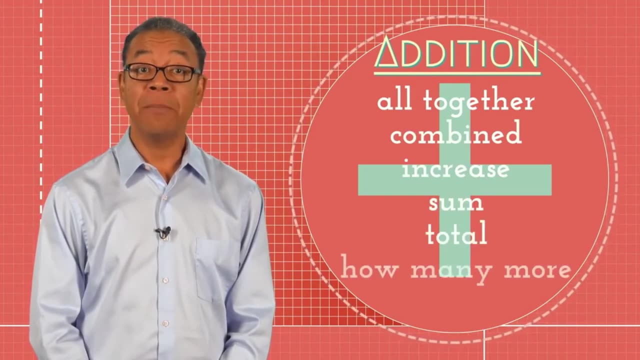 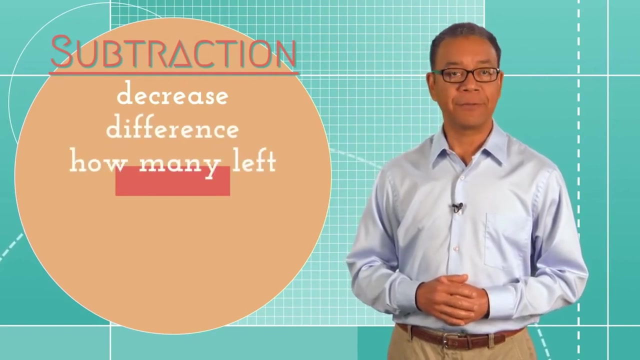 When you need to use addition, you'll likely see words such as altogether, combined, increase, sum, total and how many more. For subtraction, look for words like decrease, difference, how many left remain, take away and how many. 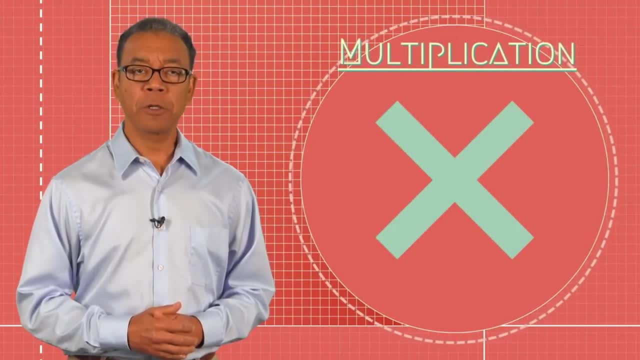 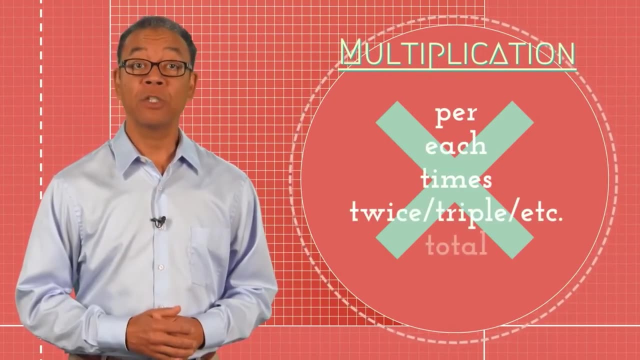 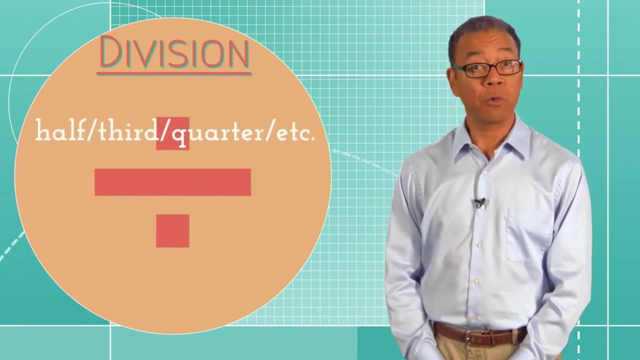 How many more then? For multiplication, you'll find words like per, each times, twice, triple, etc. and total. And lastly, for division, you'll want to keep an eye out for these words- half third. 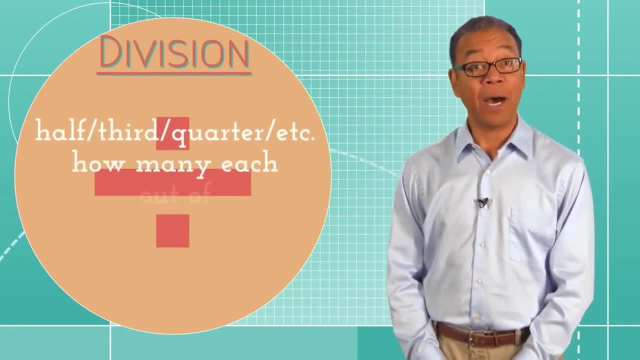 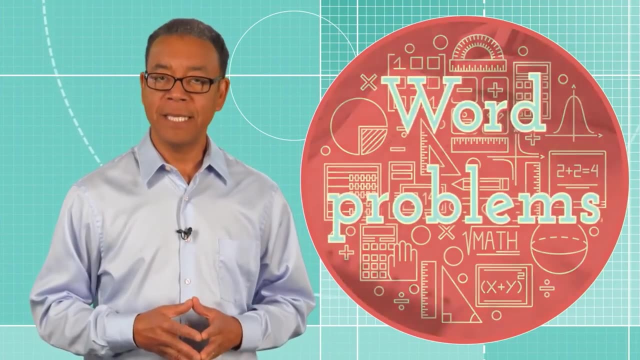 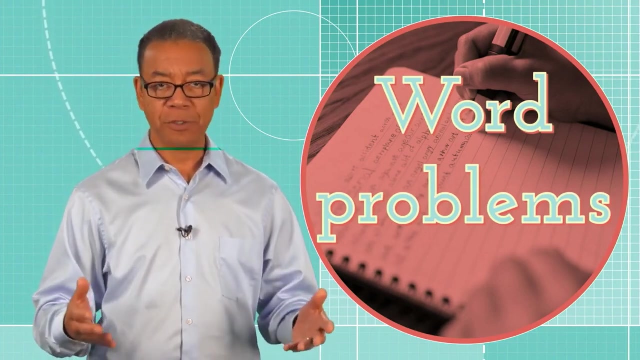 quarter, etc. How many each out of percent and quotient. Knowing how to choose the right operation is a key part of solving word problems and dealing with math in practical real-life situations. Knowing these signal words and strategies will help you successfully choose the right. 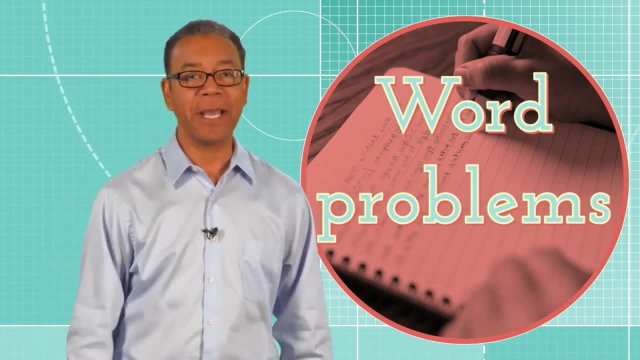 operation to solve any word problem that comes your way.